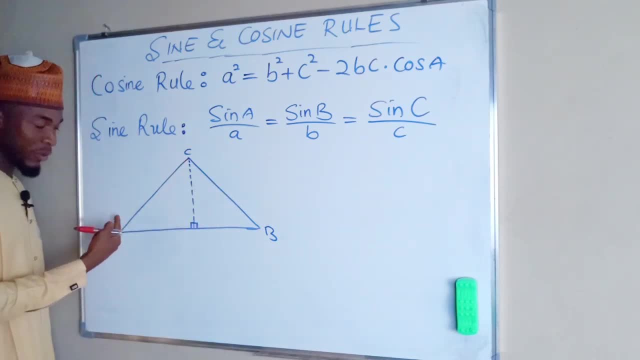 So you know that the corresponding side length to an angle will be presented a lower case later. So this is going to be A. This side length is going to be C. And, equally, this side length is going to be A. This side length is going to be a lower case later, B. 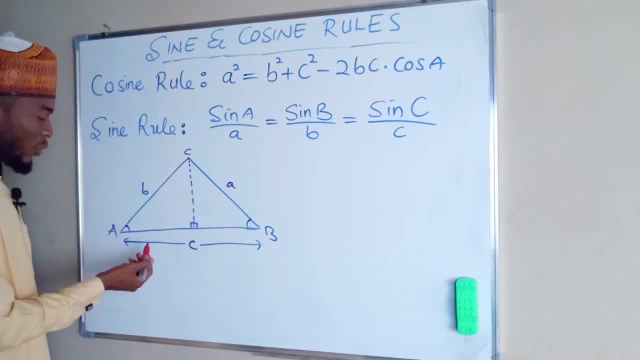 These two angles are acute angles. So if I call this side length R, let me call this place D. If I call AD as R, definitely DB is going to be C minus R. This place is going to be C minus R. Again, let us call the length CD as H. 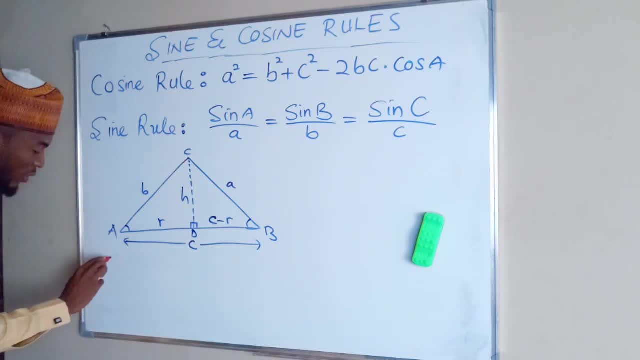 which is the height of this triangle. So let us obtain the sine of the angle A. Sine A is going to be opposite, divided by hypotenuse, and opposite is H, while the hypotenuse is B, If you multiply both sides by B. 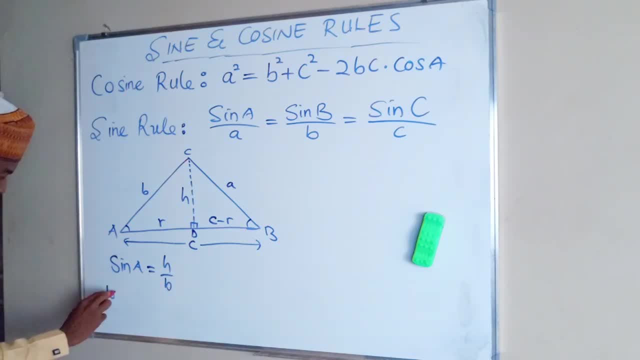 you are going to obtain B sine A equals H. Let us call this equation number one. And again we want to obtain the cos of the angle A. Cos A is going to be adjacent divided by hypotenuse, and adjacent is R. 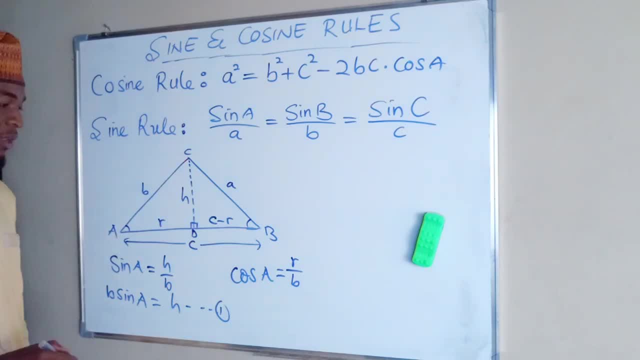 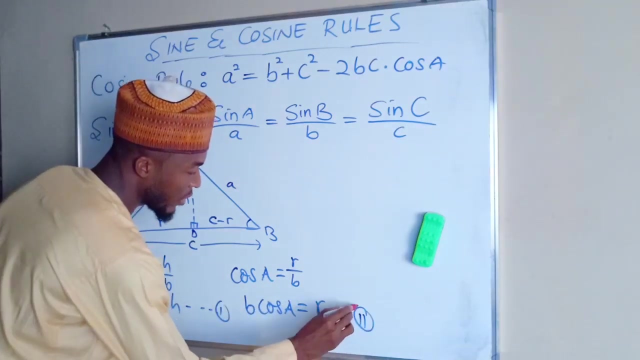 while the hypotenuse is B, the longest side of a triangle. If you multiply both sides by B, you are going to obtain B cos A equals R. Let me call this one equation number two From Pythagoras' theorem. it says: hypotenuse squared is equal to: 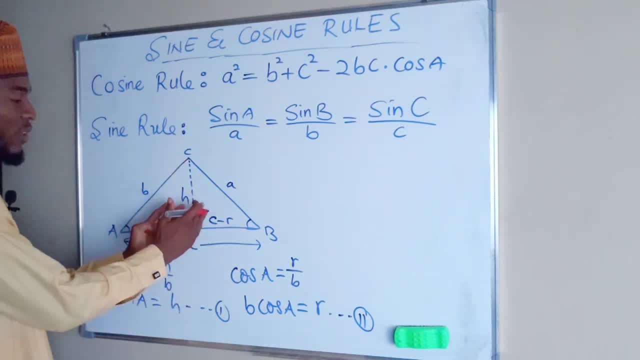 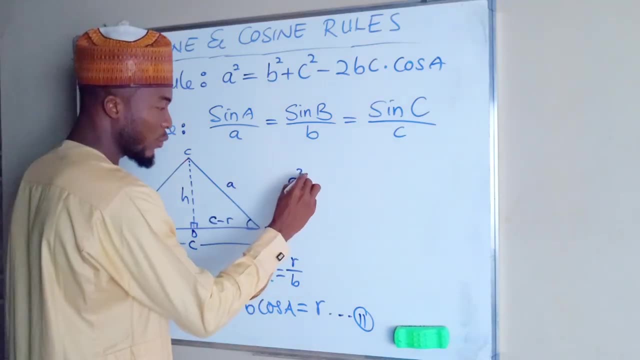 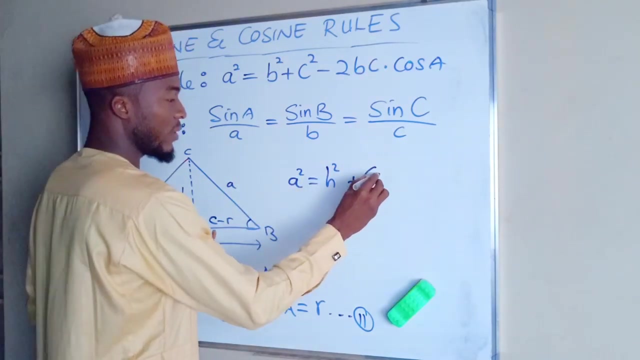 opposite squared plus adjacent squared. So let us use the other triangle, which is triangle CDB. The hypotenuse there is A squared equals to the opposite squared, which is H squared plus the adjacent, which is C minus R, also squared. 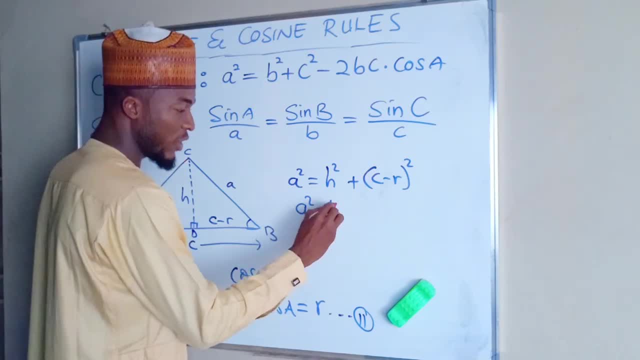 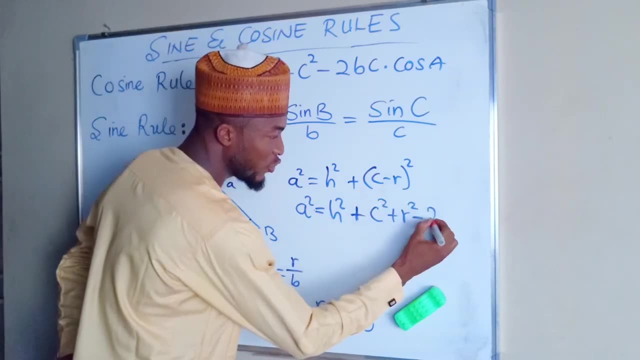 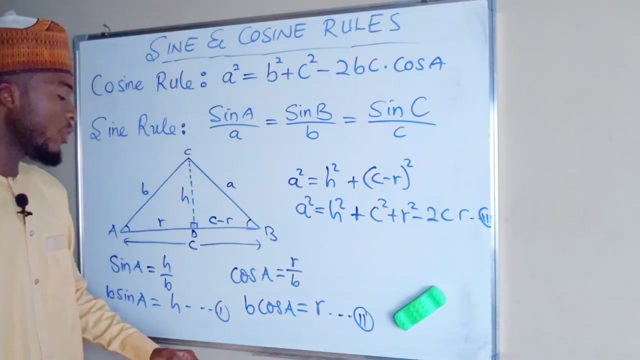 A squared equals H squared. If you expand this, you are going to obtain C squared plus R squared minus 2CR, equation number three. So what we are going to do now, we are going to substitute equation one and equation two into equation number three. 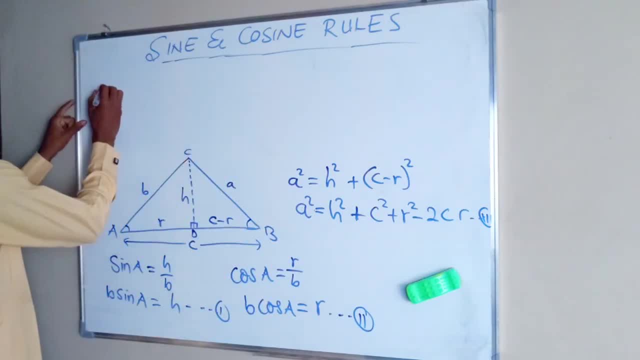 From equation three we have the first term from the left-hand side equals to A squared. This is equal to: we have H squared. From equation one: H equals to B sin A. So we replace H with B sin A, B sin A squared. 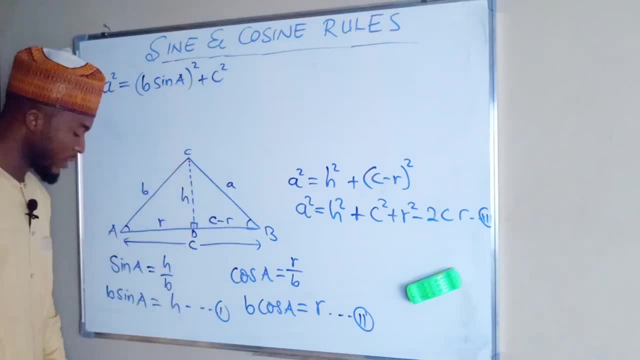 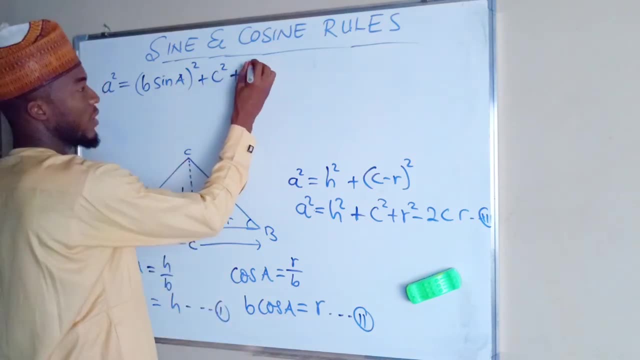 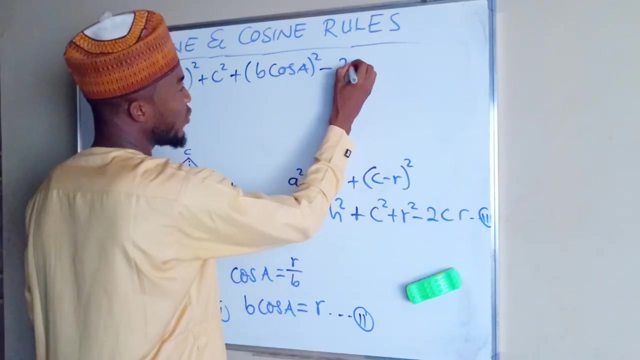 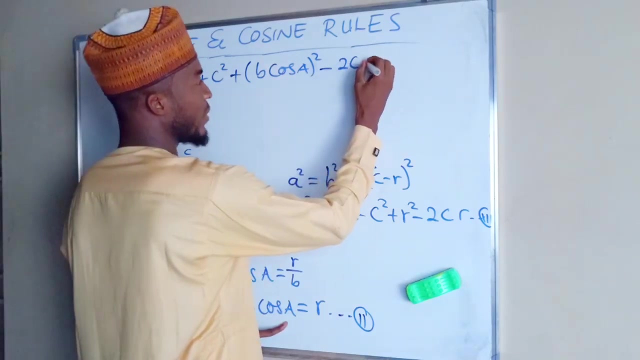 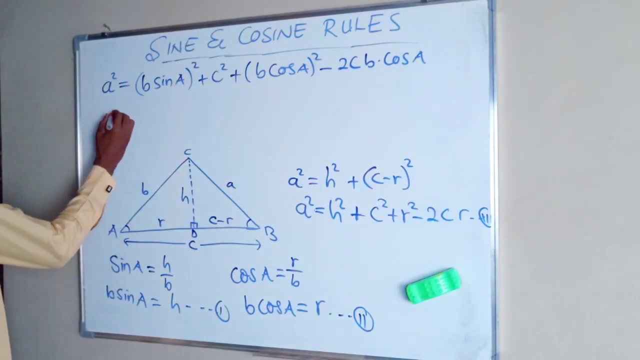 Then plus C squared plus R, We have from equation two R equals to B cos A, B cos A, also squared, Then minus two times C, times R, but R is given as B cos A. So we have B cos A. A squared is equal to. 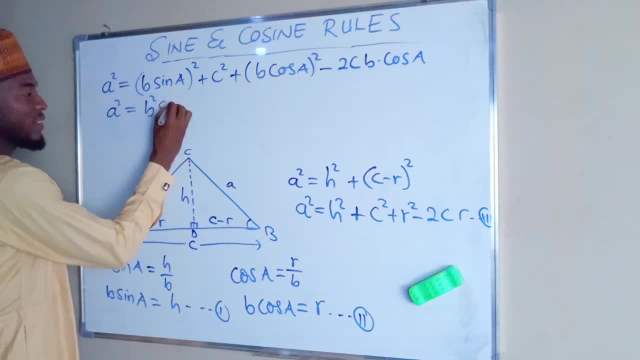 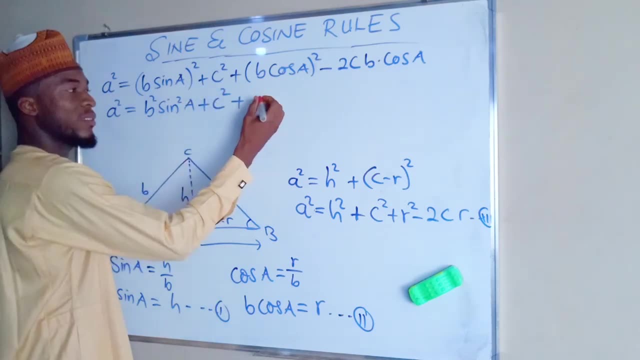 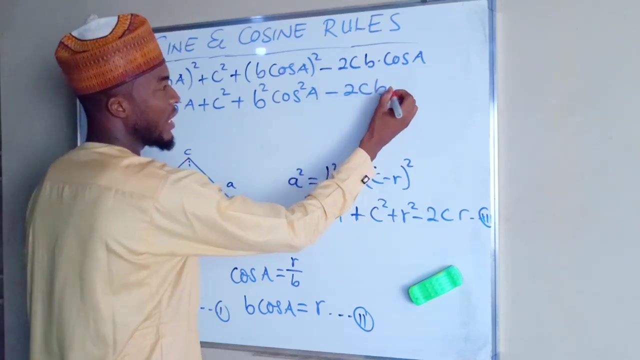 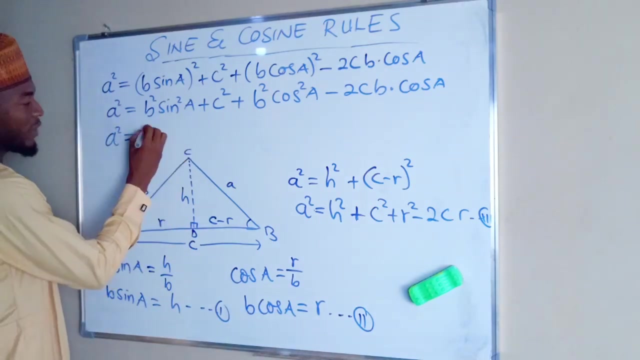 if you expand this, you are going to obtain B squared sin squared A, plus C squared plus. if you expand this, you are going to obtain B squared cos squared A. then, minus two C, B times cos A, A squared will be equal to B squared sin squared A. 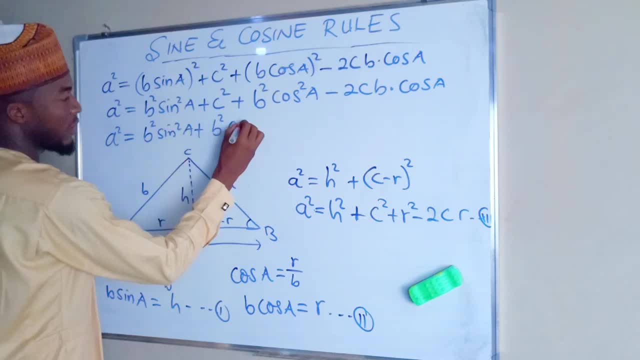 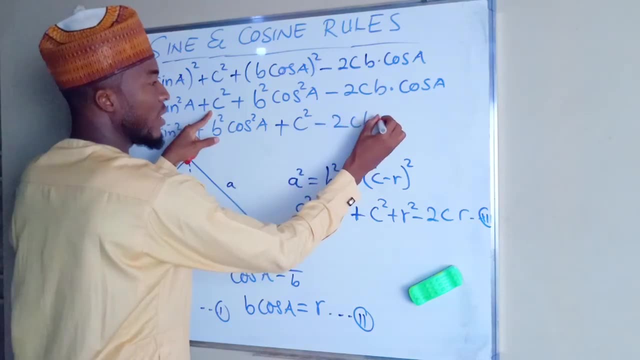 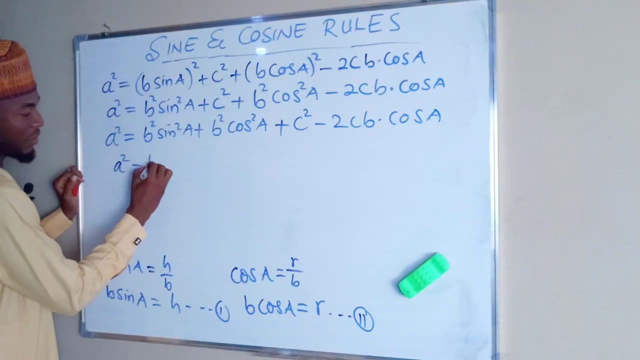 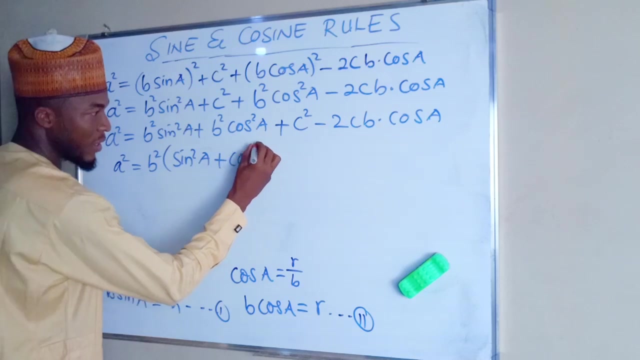 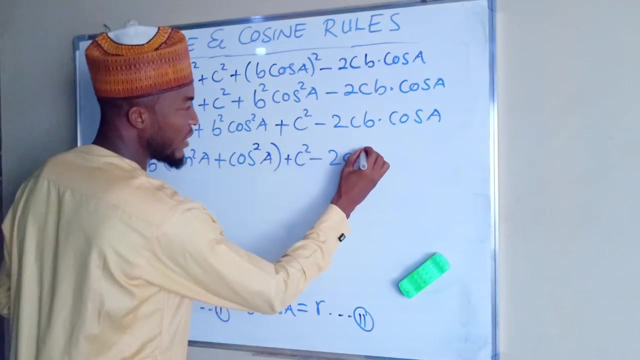 Then plus B squared cos, squared A plus C squared minus two, C, B cos A. By factorization this is going to be B squared in the bracket of sin, squared A plus cos squared A. Then plus C squared minus two, C B cos A. 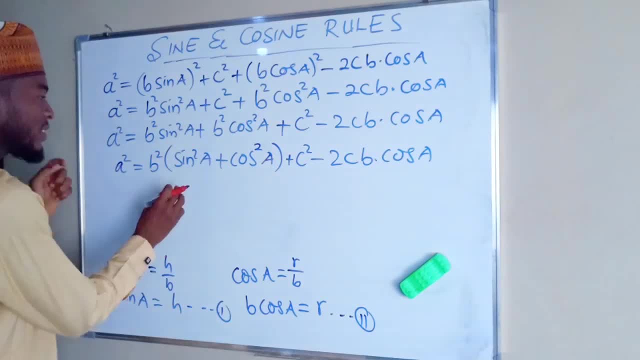 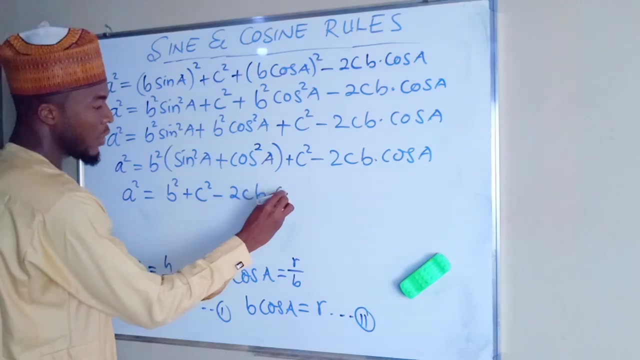 Then plus C squared minus two C, B cos A. From trigonometric identities you know that sin squared A plus cos squared A is going to give us a. one A squared is now going to be B squared times one is B squared plus C squared minus two C, B cos A. 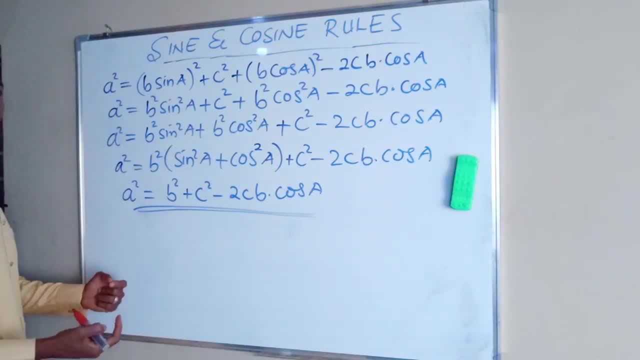 The cosine rule. If you are looking for a sideline of B, you are going to say B squared equals to A squared plus C squared minus two. C, B cos A. If you are looking for a sideline of C, you say C squared equals to. 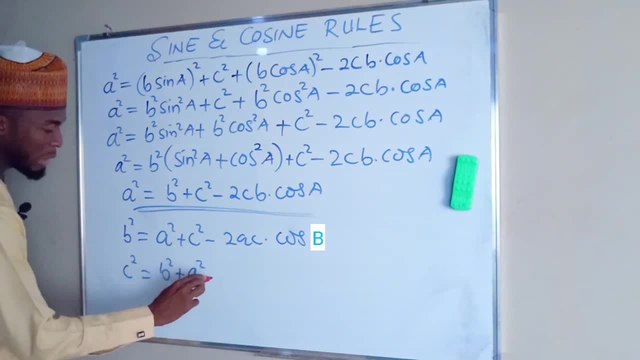 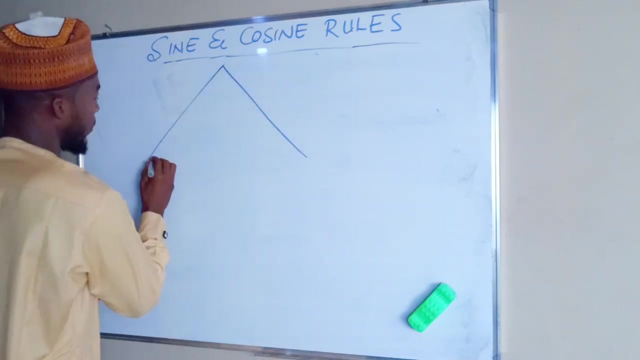 B squared plus A squared minus two B, A cos C. Then for sin rule, Suppose we have a triangle this form: If you draw a line from C perpendicular to the line AB, you are going to form two right angle triangles. So let us call this length H. 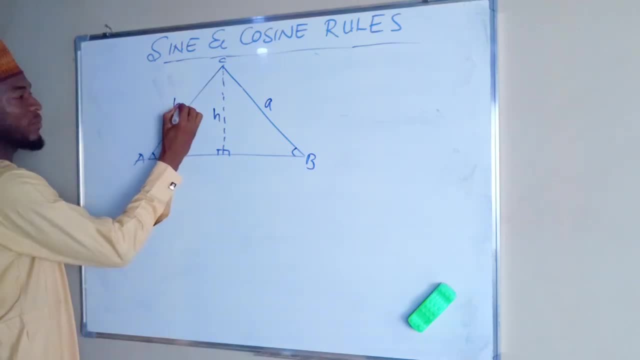 This is going to be A, While this is going to be B. Sin A is going to be opposite, divided by hypotenuse, H divided by B. If you times both sides by B, you are going to have H equals to sin A times B or B sin A. 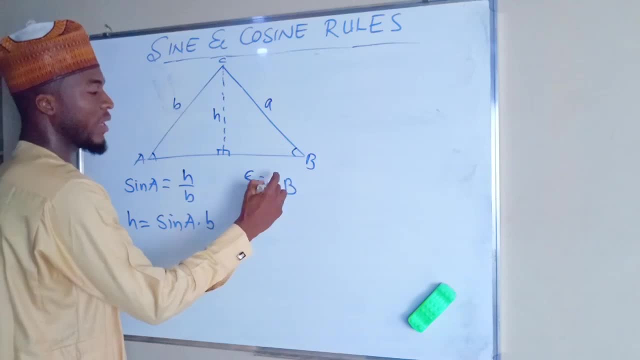 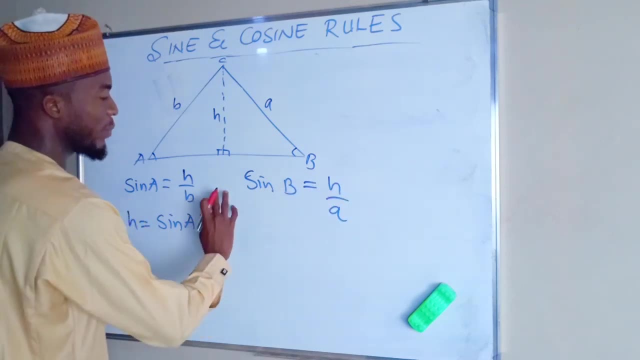 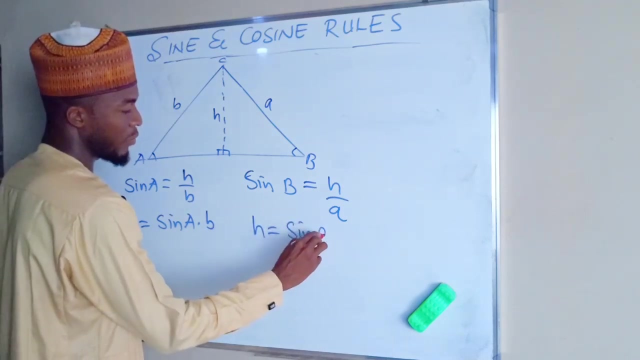 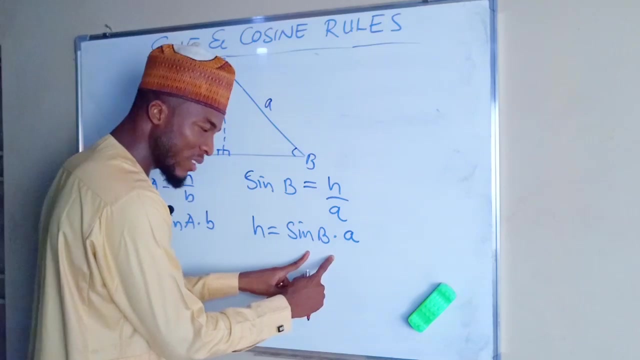 Then sin B, Sin of B, is opposite. divided by hypotenuse, This is H divided by A. If you multiply both sides by A, you are going to obtain H equals sin B multiplied by A, Since H equals to this and H equals to this. 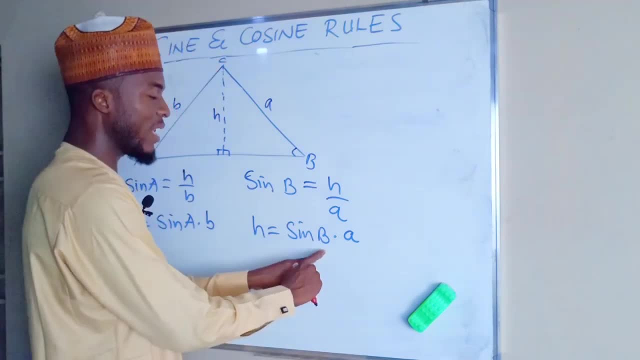 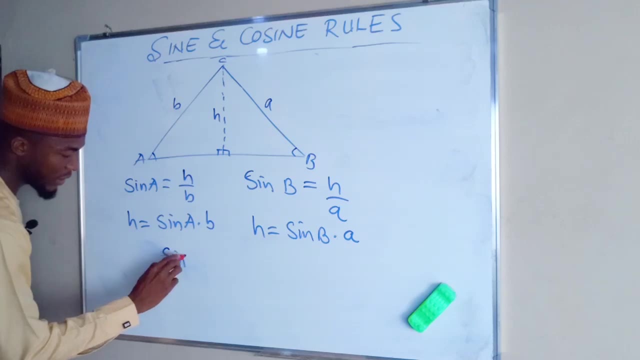 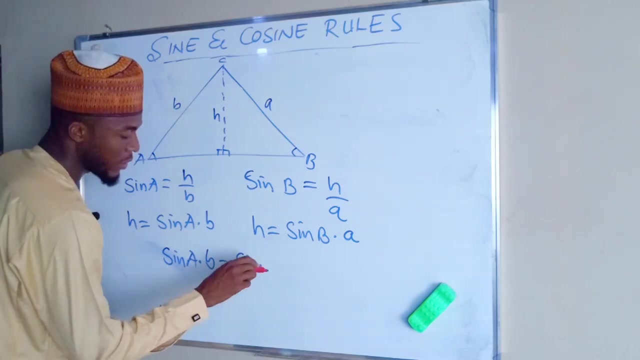 this means that sin A times B is the same thing as sin B times A, Because all of them equals H. Therefore, we compare the two: Sin A times B equals sin B multiplied by A. Now what we are going to do is to divide each of these sides by AB. 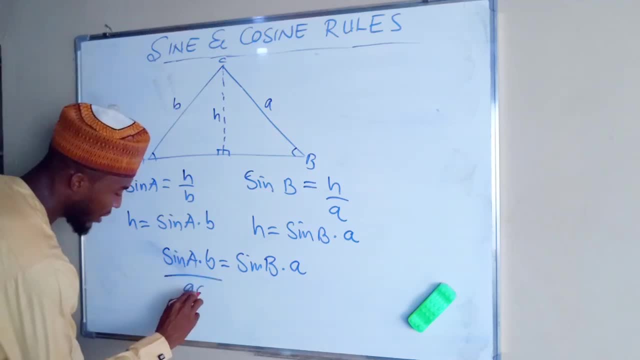 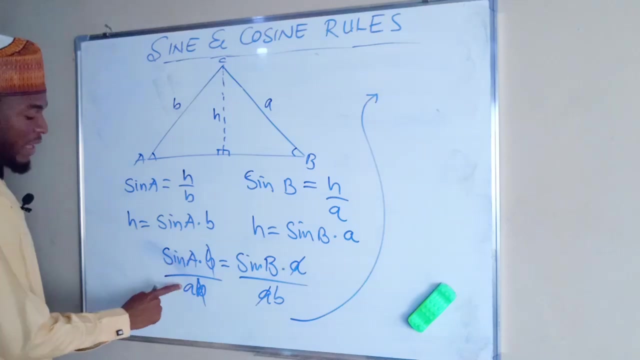 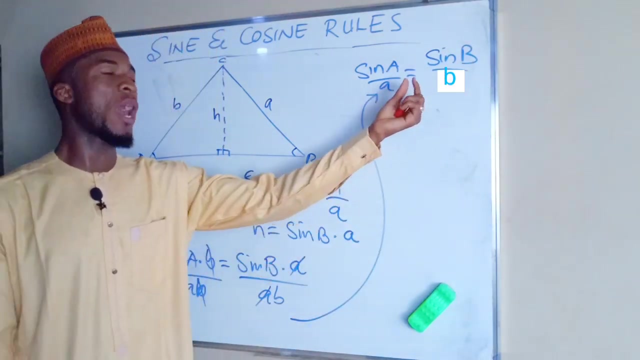 So we divide both sides by AB. This A cancels this And this B cancels this. We end up having sin A over A equals sin B over B. We don't have for angle C, But if you draw a line from A perpendicular to the line CB,